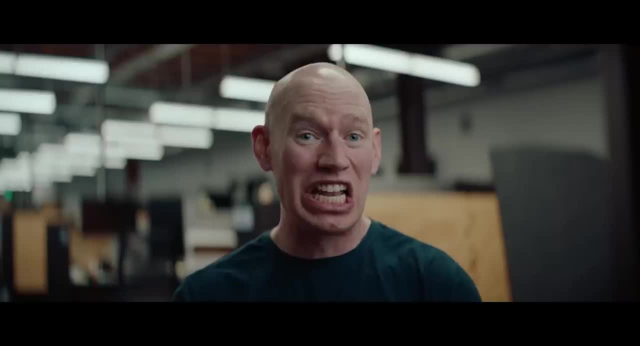 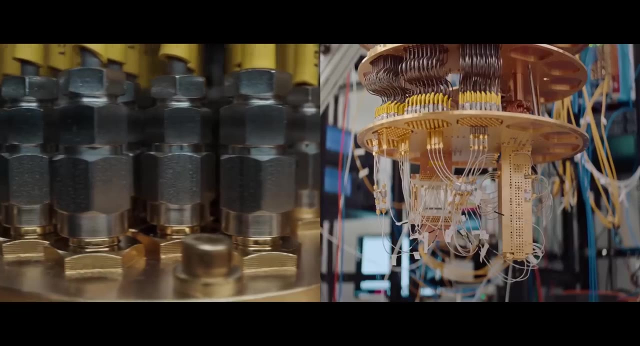 In order to make this experiment work, a lot of things have to work at the same time: The quantum chip, all the qubits, the fridge and the electronics and the cables and everything, And so there's a lot of trial and error that goes into getting all this hardware working together. 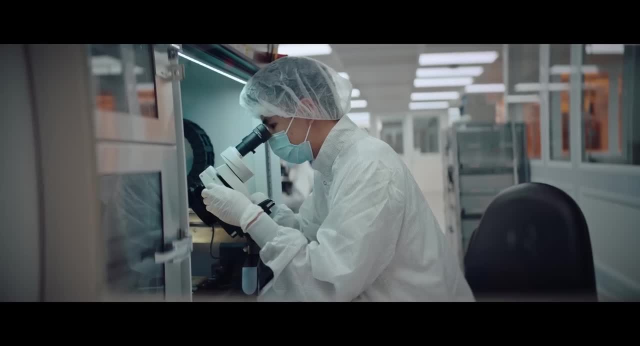 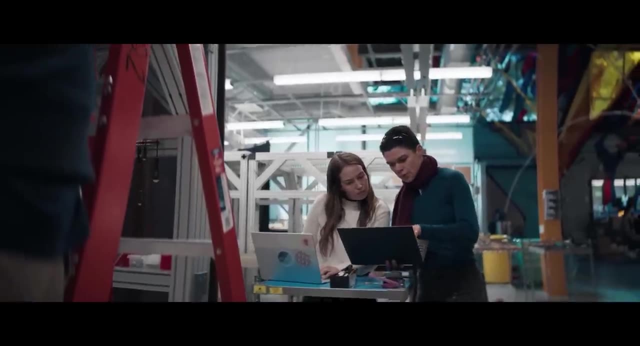 It just kept cranking over a period of months And at some point we thought we could really attempt the experiment fully for the first time. But then when we actually go to run the algorithm, their performance was terrible- The sophistication of the system and what we were trying to do with it. were beyond anything that we had ever done before, And so we basically had to develop a new language that we used to make the chip do what we wanted it to do, And that took a lot of hard work from a lot of very smart and dedicated people. 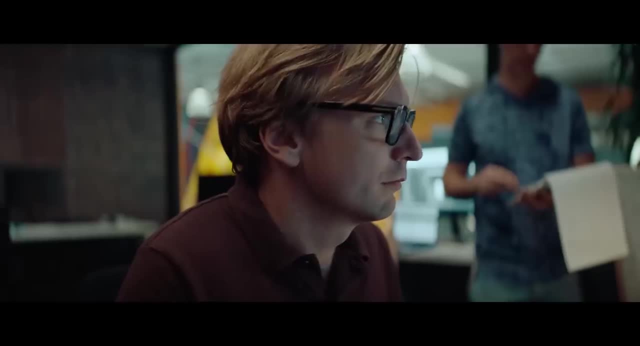 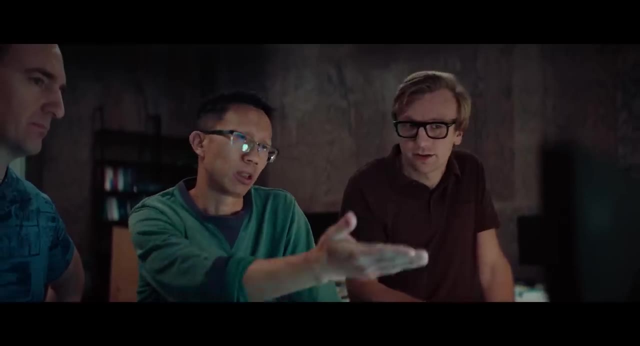 Communicating with the qubits is pretty tricky because we don't want them to interact with the environment on accident, but we do want them to listen to the signal that we're sending to them And it's not just telling the qubits what to do. 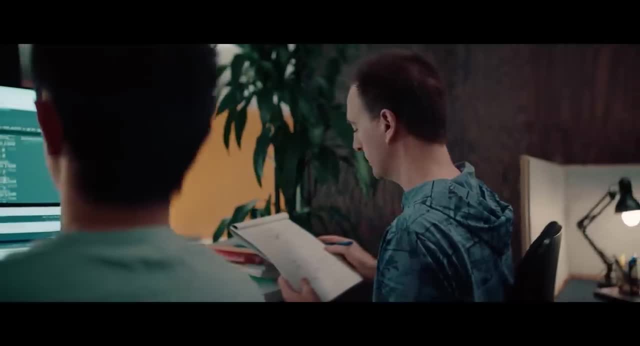 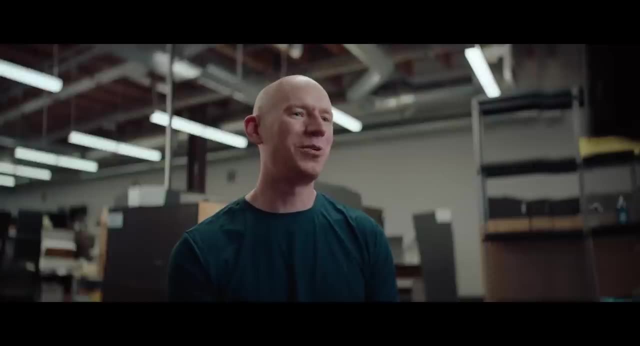 We also need to get information back from the qubits so that we can ask what state were you in At the beginning. even though the errors were pretty high, I felt like you know, we can grind this out, We can make it happen. 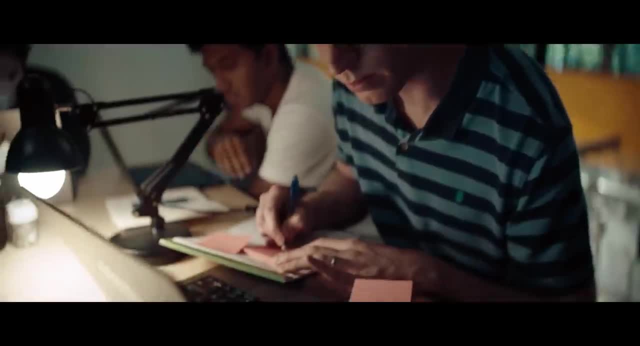 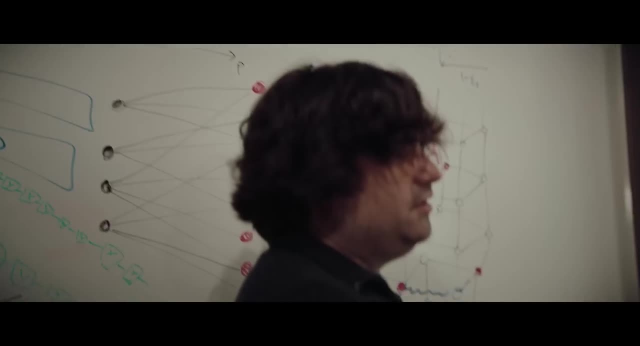 There were a lot of people on the team who were figuring out new ways to make the operations better, new ways to make our decoding better. Is there another decoder that can get us there, Maybe After a few months? it was definitely like weighing on us. 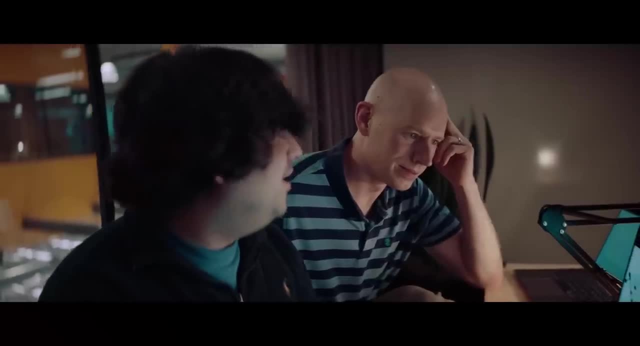 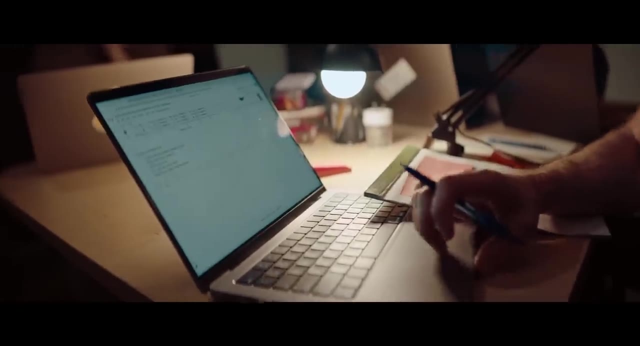 Like, oh gee, maybe this isn't actually going to work. I'd certainly say that resilience is strong on this team. Not everyone has the same approach to solving. It's not always about solving a particular challenge. When progress slows, you start to worry, you know. 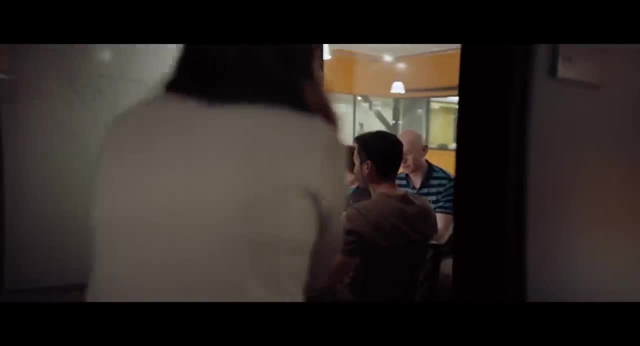 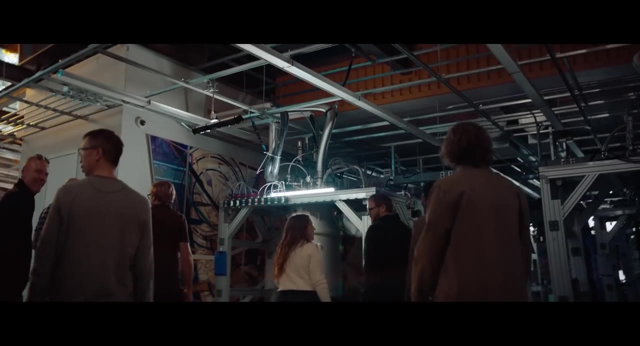 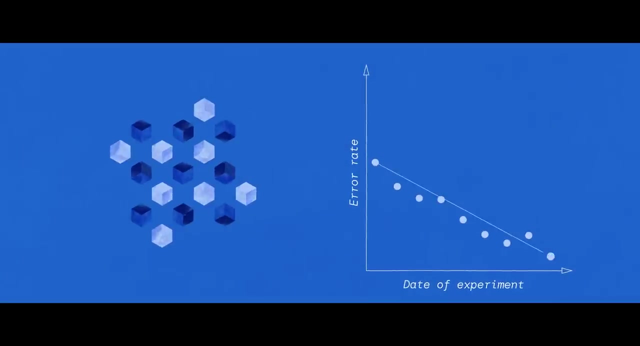 will we ever get there? We're pushing on the experiment, we're pushing on it, we're pushing on it, and then, finally, it just clicks. For the first time, we have gone past the break-even point, Even though we went to a larger array of data- qubits. 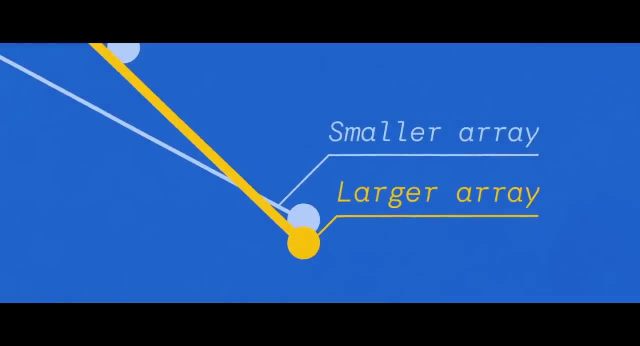 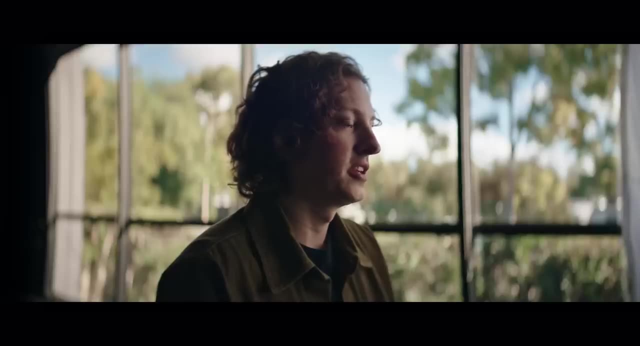 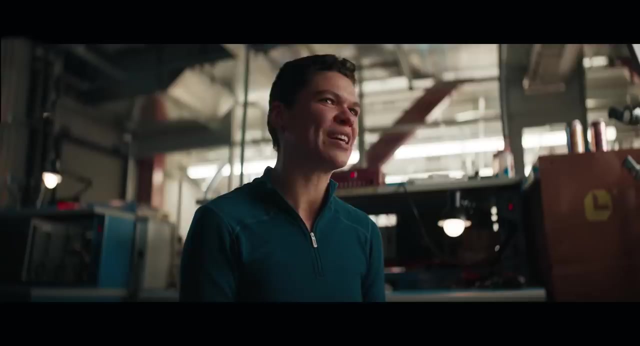 the error rate came slightly down. We showed that quantum error correction doesn't only work in theory, but that it actually works in practice. And what that does is it opens the door towards making very large and powerful quantum computers in the future. I am optimistic that, equipped with a quantum computer